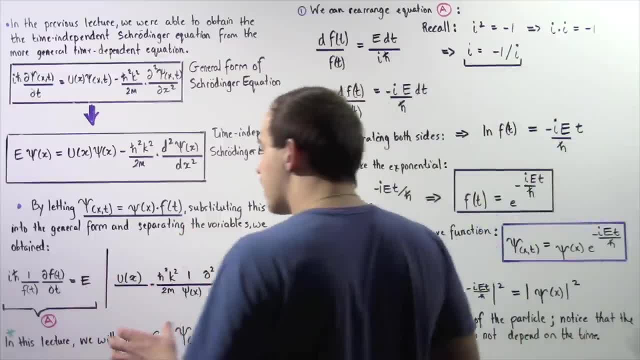 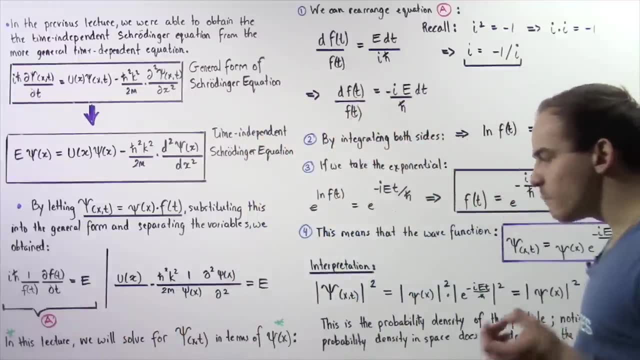 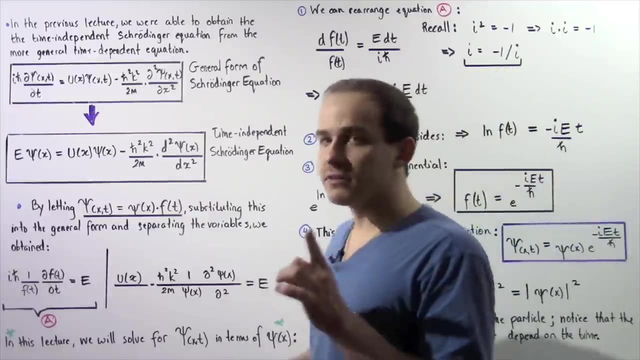 right side has a second variable. And then we ended up with the following two equations where e is simply some arbitrary constant. Now, if you're not certain what I just said, go back to the previous lecture and review what we did in that lecture. Review what we did. 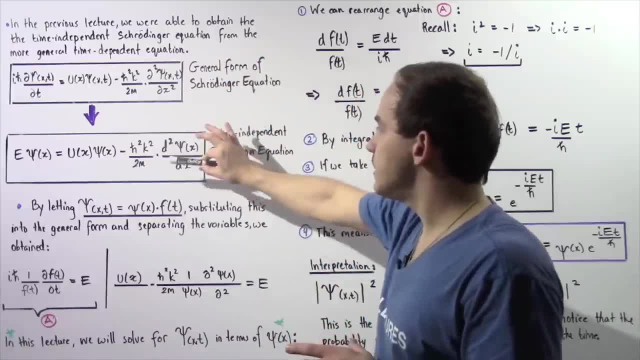 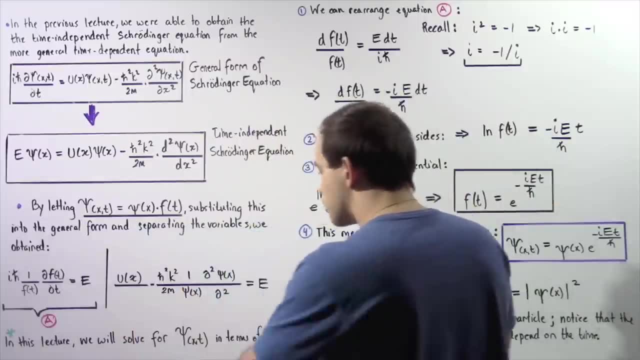 specifically to get from this general form to this specific case. So in the previous lecture we basically focused on the following equation: So we took this equation. we multiplied the left and right side by our side. So we took this equation, we multiplied the left and right side. 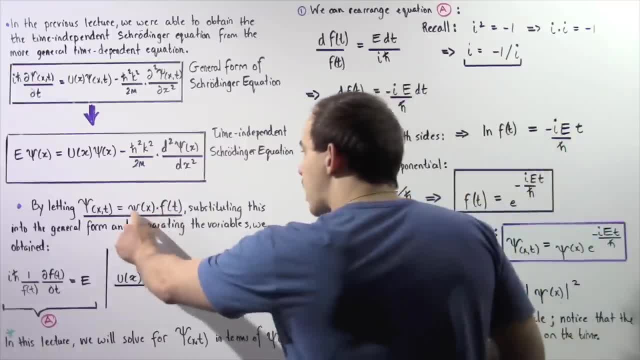 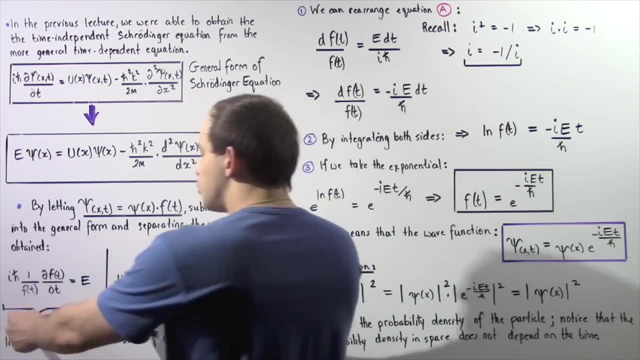 by our side. So we took this equation, we multiplied the left and right side by our side With respect to x, this quantity, and we ended up with this equation. But in this lecture our focus will shift onto the following equation. So e, our arbitrary constant. 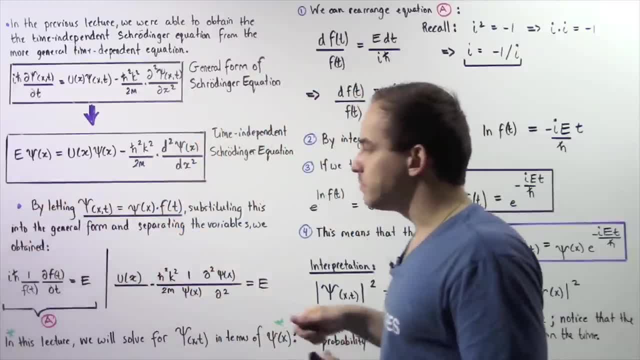 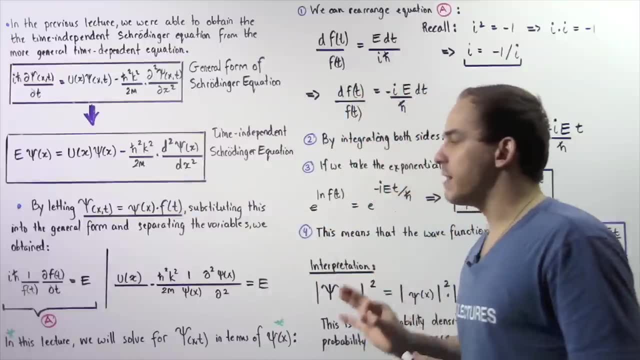 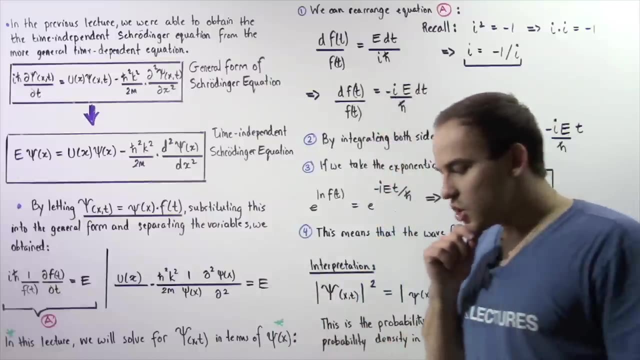 is equal to i multiplied by h bar multiplied by 1, divided by f of t, multiplied by our derivative of f of t with respect to time. Now, what exactly will be the focus of this lecture? What will be our goal? So we basically want to take the following equation, which we're going 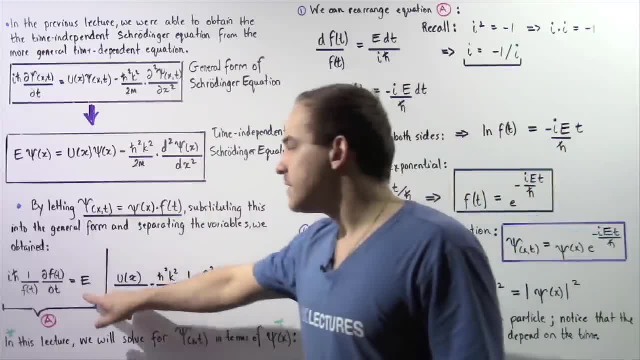 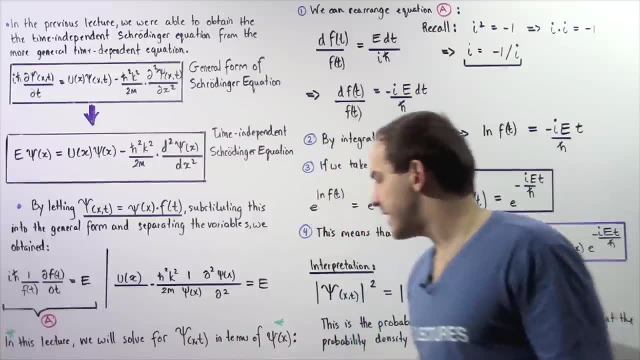 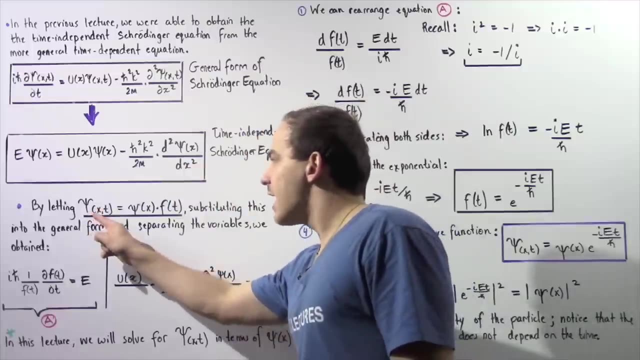 to label as equation a And we're going to solve this equation. We're going to try to determine an equation for the total wave function in terms of our wave function. So we want to determine our equation for psi x comma t, with respect to only lowercase psi x. 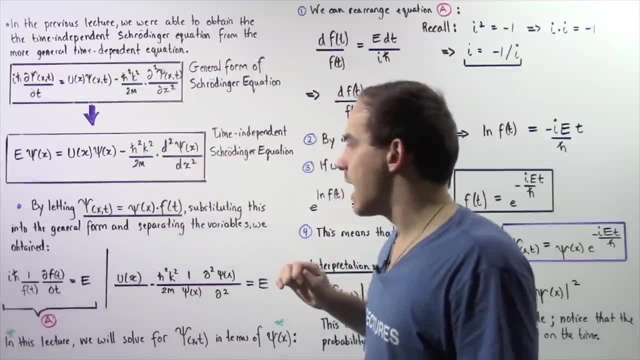 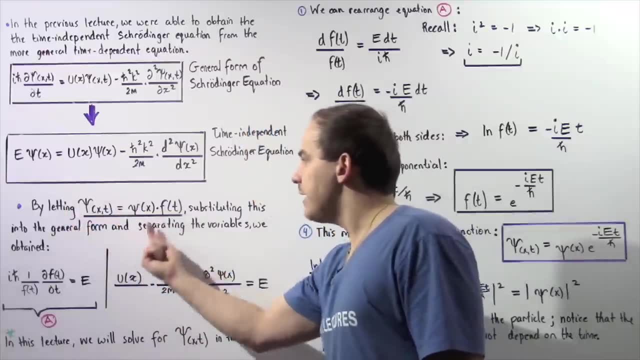 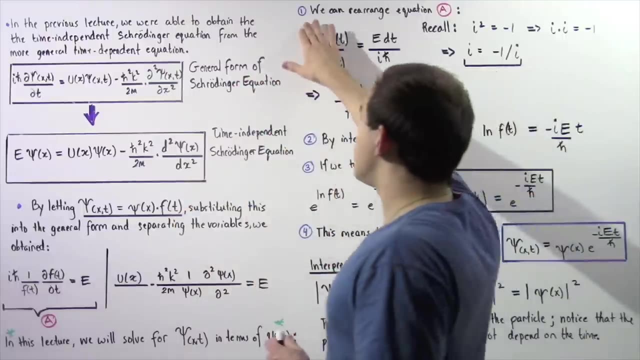 uppercase side, by the way, and this is lowercase side. We use uppercase and lowercase to distinguish between the total wave function and our wave function. that appears in the time-independent Schrodinger equation. So let's begin with step one. We basically have four steps that we're 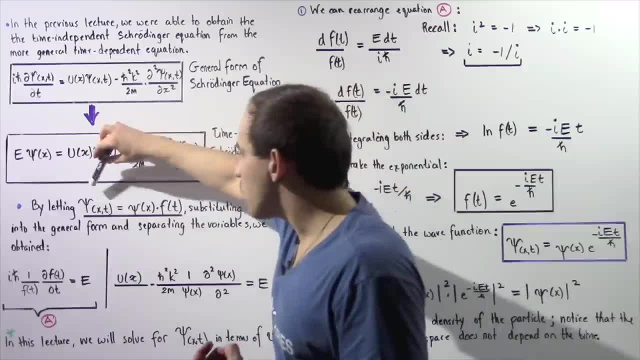 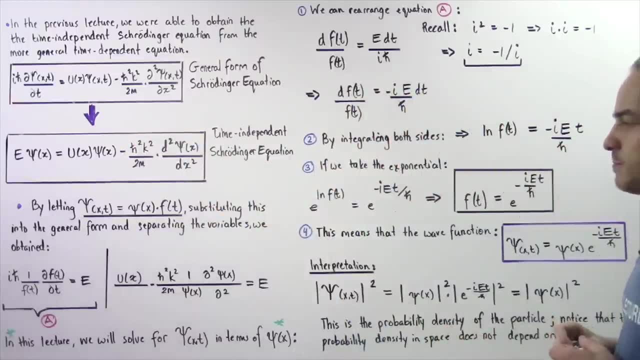 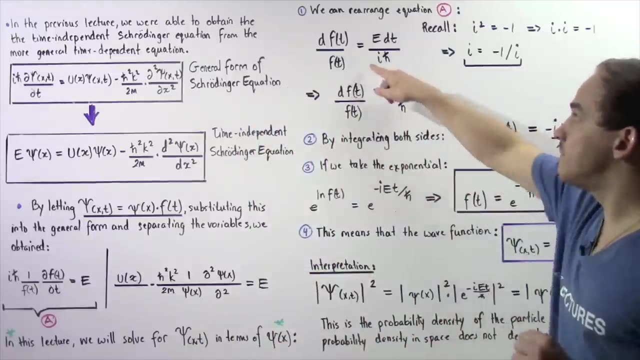 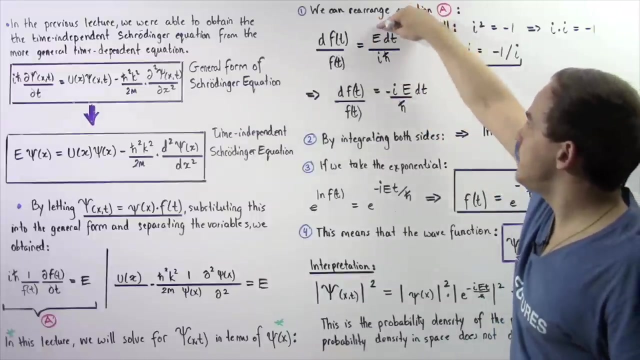 going to follow to determine an equation for our total wave function with respect to our wave function. So let's begin with equation A and let's take equation A and let's rearrange equation A as follows: So the left side- we have d, f of t divided by f of t is equal to e. 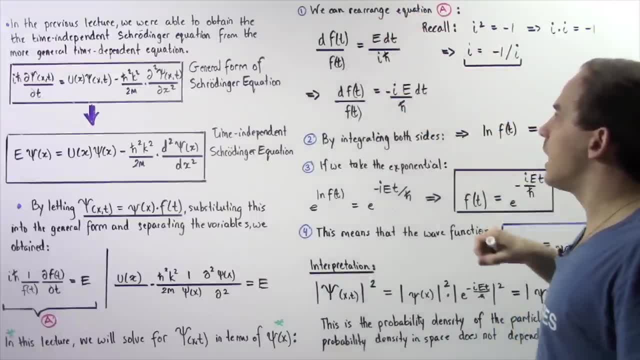 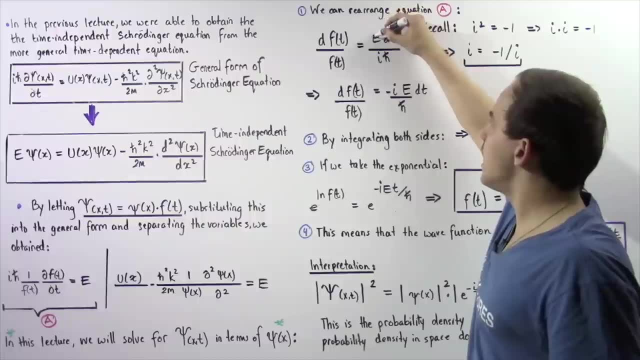 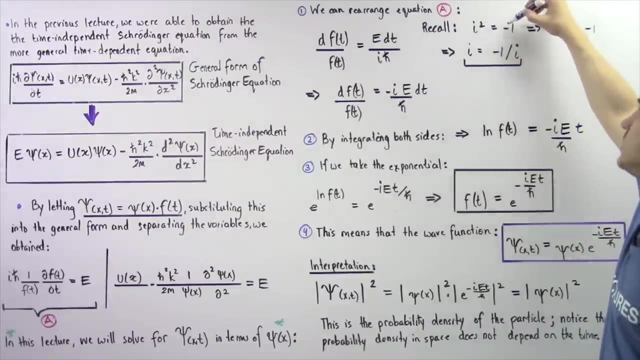 multiplied by dt, divided by i, multiplied by h bar. So now we basically want to take our i and we somehow want to bring the i to the numerator, which is the term of this equation. Now, recall that i squared is equal to negative one. Now, 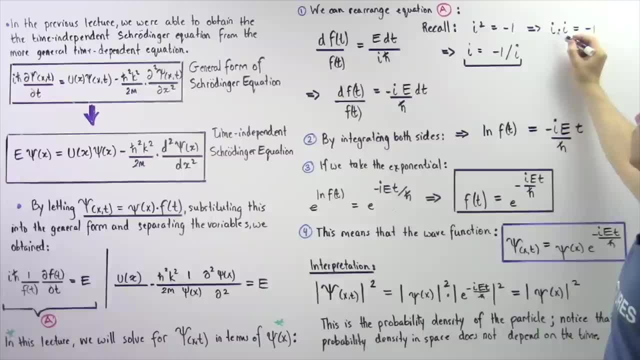 another way to represent i squared is simply multiplying i by i. So i squared is equal to i multiplied by i, which is equal to negative one. Now, if we divide both sides by i, one of these i's will cancel and we see that another way to represent i is simply negative. 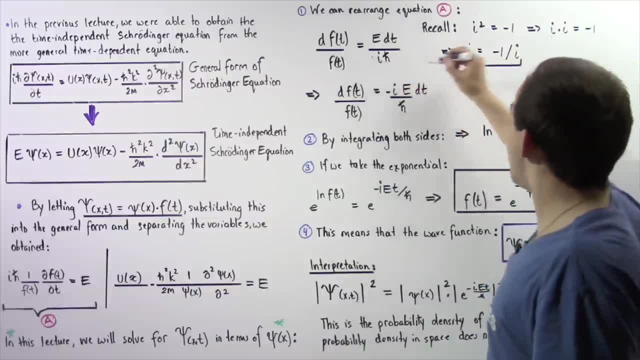 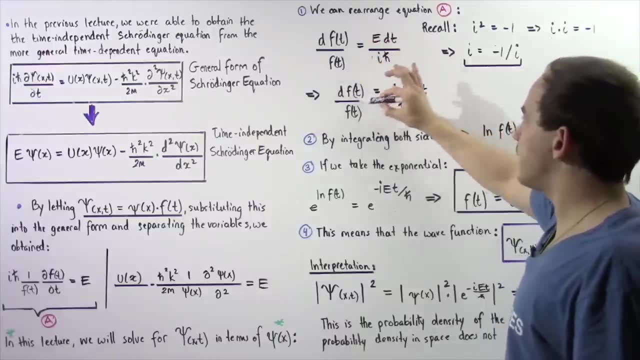 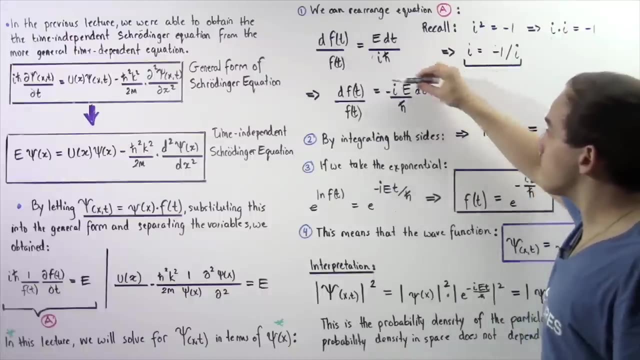 one divided by i. So if we replace this i with negative one divided by i, we get the following equation: So d? f of t divided by f of t is equal to negative. i e dt divided by i. bar Now d f of t is simply: 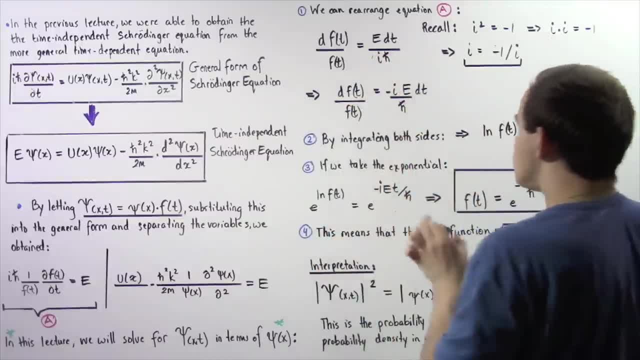 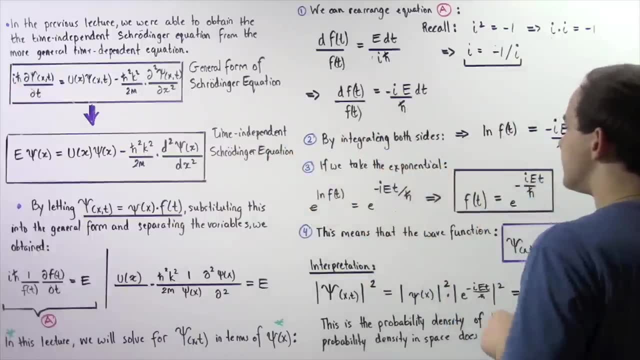 an infinitely small quantity, and dt is also an infinitely small quantity. So we can now basically integrate both of these sides. If we integrate the two sides, we're going to get the following result: If we take the exponential of the left side, we get natural log of f of. 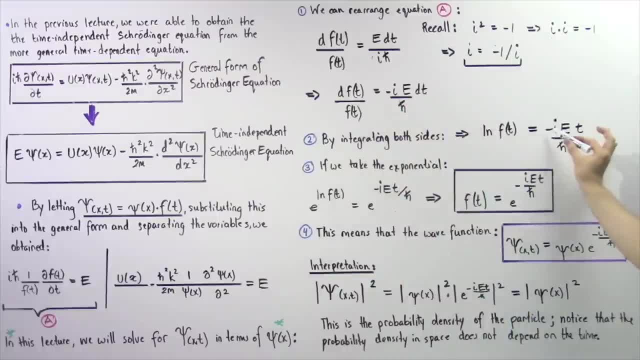 t. If we integrate the right side, we get negative i multiplied by e, divided by h bar, and this dt simply becomes t. So now let's take this equation and move on to step three. So now we basically want to take the exponential of the left and right sides. So if we take 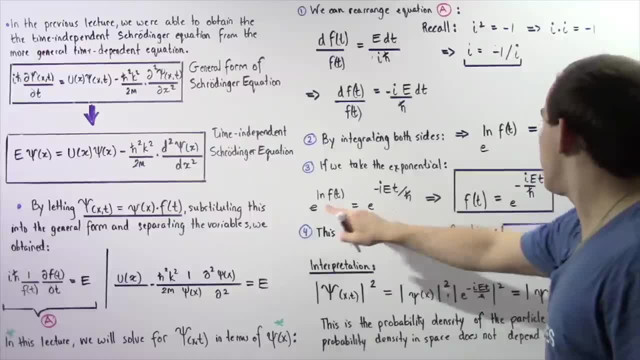 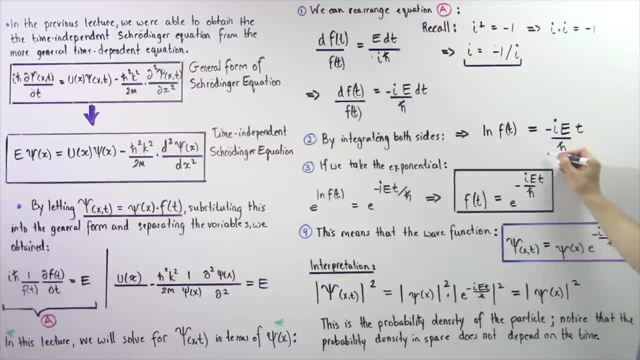 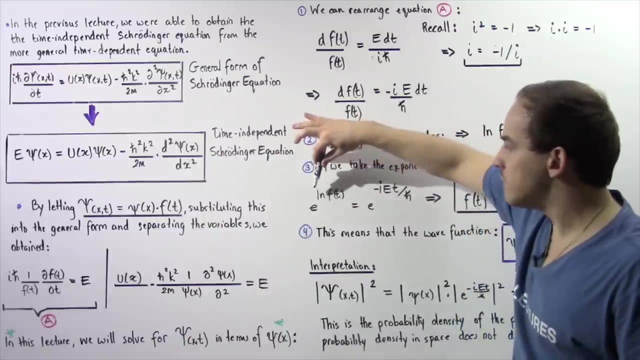 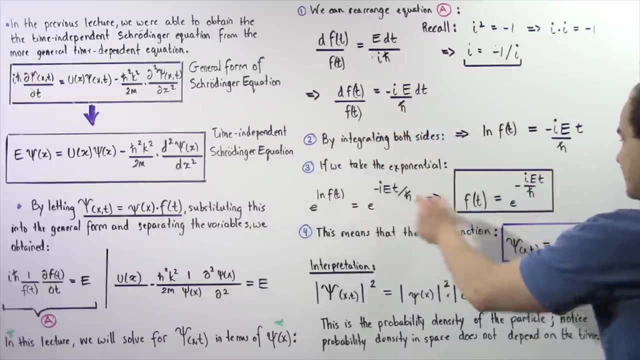 the exponential of the left side, we get the following result: Now notice that the exponential e to the power of ln is simply f of t. So we see that f of t is equal to e to the power of negative i multiplied by e, multiplied by t divided by. 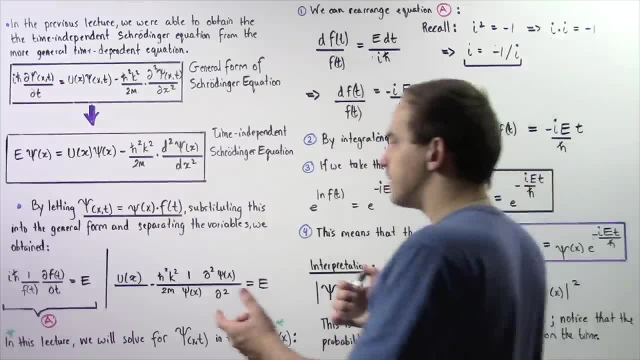 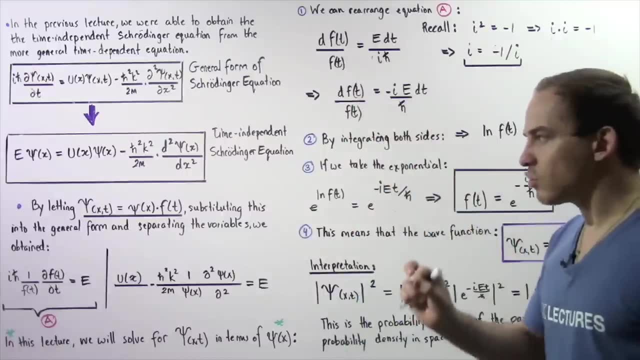 h bar. So now we are ready to go back to the following equation. So now we are ready to go back to the following equation and replace f of t with the following result. So remember, our goal was to basically take the total wave function that appears. 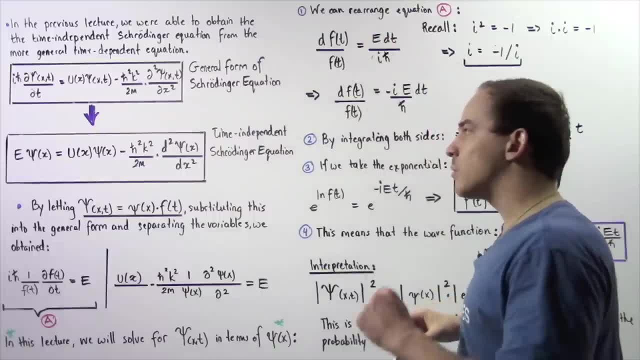 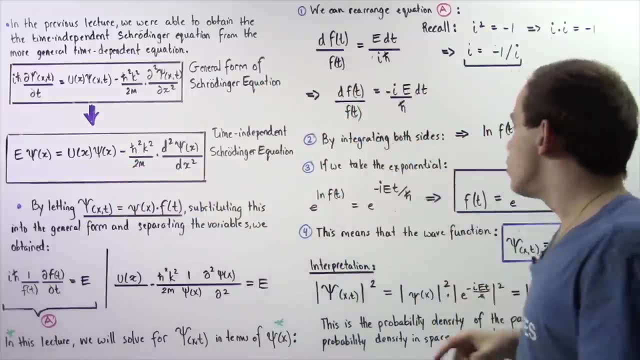 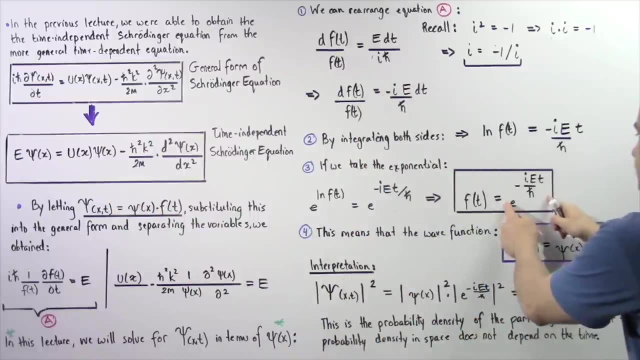 in the general form of the Schrodinger equation and represent it using our wave function that appears in the time-independent Schrodinger equation. So we basically take this equation and we plug in this exponential quantity. So we see that the total wave function that depends on position and time is equal to the. 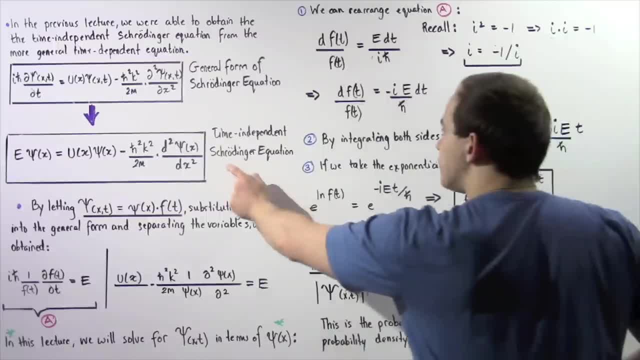 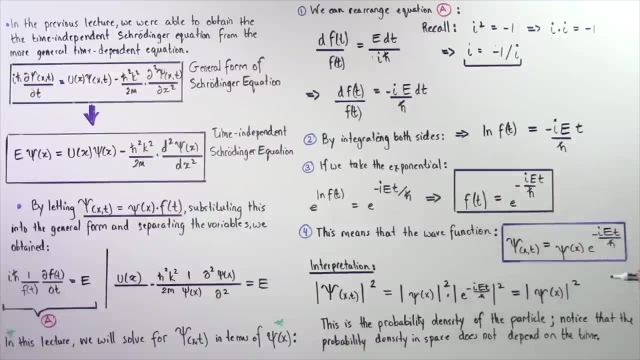 wave function that only depends on the position that appears in the time-independent equation, multiplied by f of t, which is equal to this quantity e to the power of negative i, multiplied by e times t divided by h bar. So what exactly is this? What is the meaning of this equation? 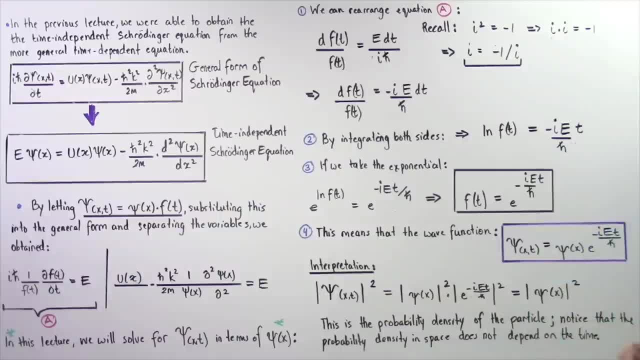 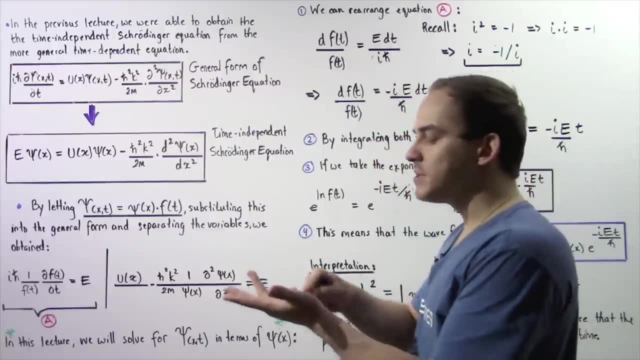 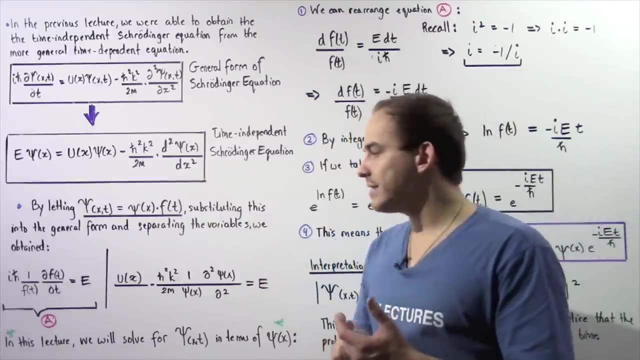 So let's try to interpret what this equation actually means. So we basically determine the equation for the wave function that depends on position and time. in terms of the wave function, that only depends on the position and does not depend on the time. Now the question is: what is the meaning behind this equation? 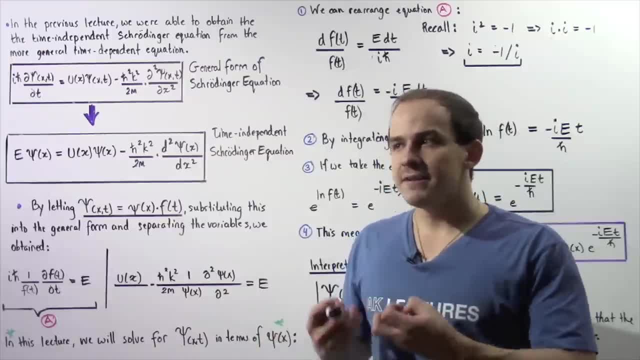 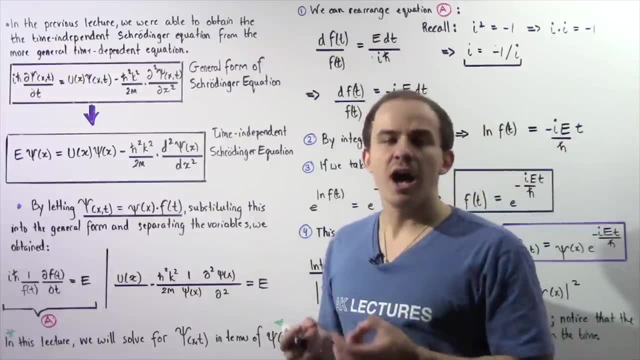 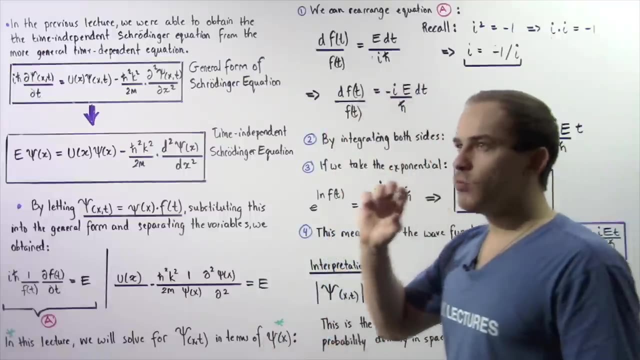 Well, what is the wave function? The wave function, The wave function, gives us a way that we can represent the motion and behavior of any object on the atomic and subatomic level in quantum mechanics, such as, for example, an electron. So when an electron moves along the x-axis, we can describe the motion and behavior of. 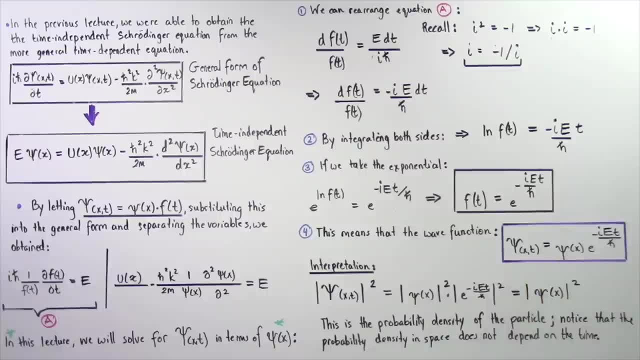 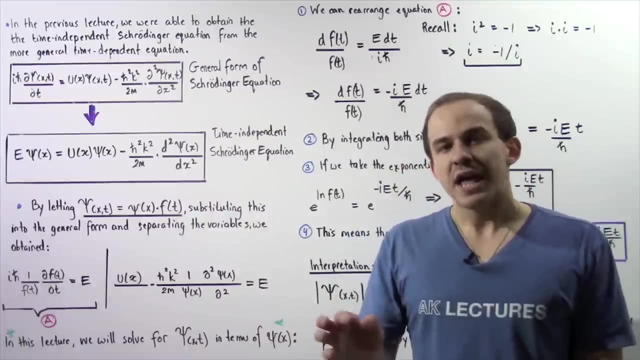 that electron as it moves by using this equation. Now notice that this equation has a negative i term. It has an i. And what exactly is the i? Well, the i is basically an imaginary number. It's a number that does not actually exist. 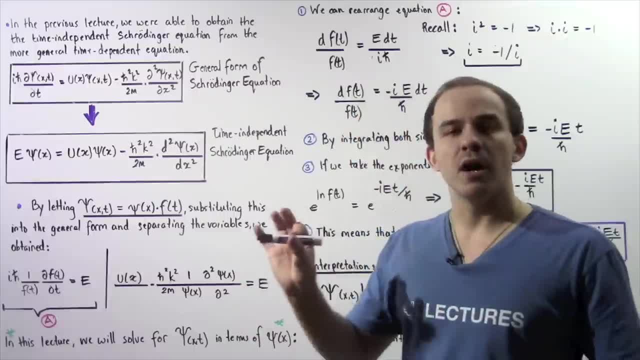 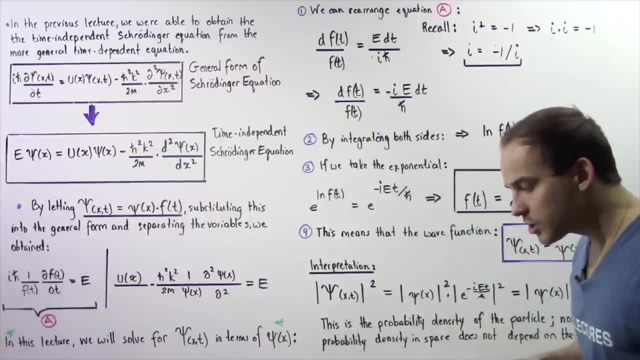 So we can simply say, for example, that we have i number of markers, because i is a number that doesn't exist. We can say we have one, two, three, four number of markers, but we can't say we have i number. 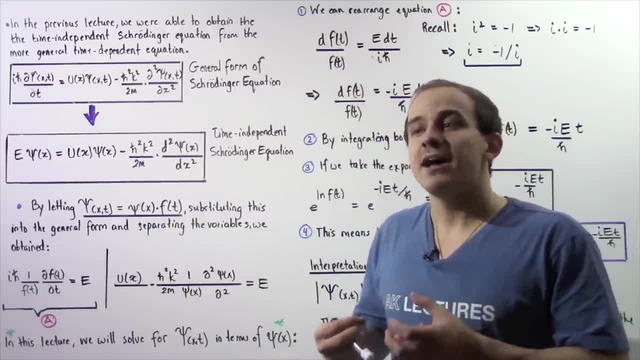 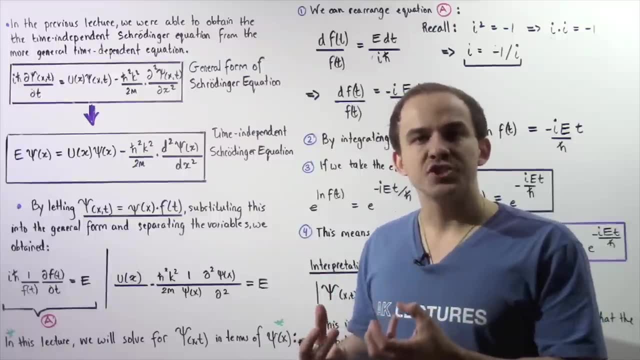 of markers. So that basically means i is not a real number in the sense that it is not a real number. So the i is a number, The i is a number, The i is not physical measurable. We can't actually visualize what the number i means. 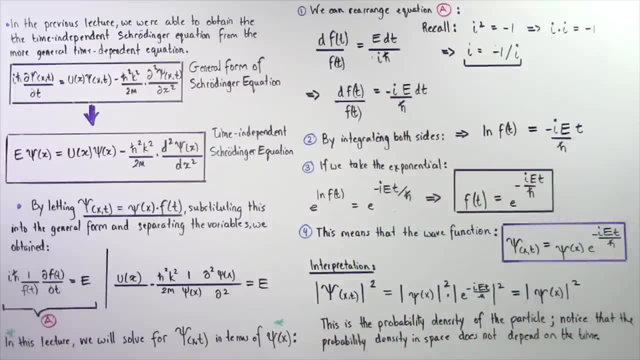 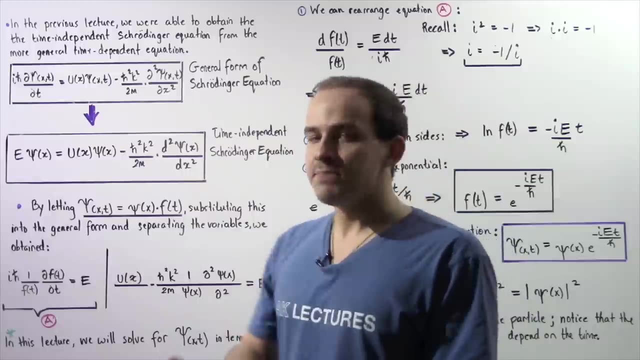 Because the i appears on the right side of this equation. that means we cannot actually measure what the wave function is. Our wave function in this term, in this form, is not actually physically measurable. It's not actually physically meaningful If we somehow take this function. 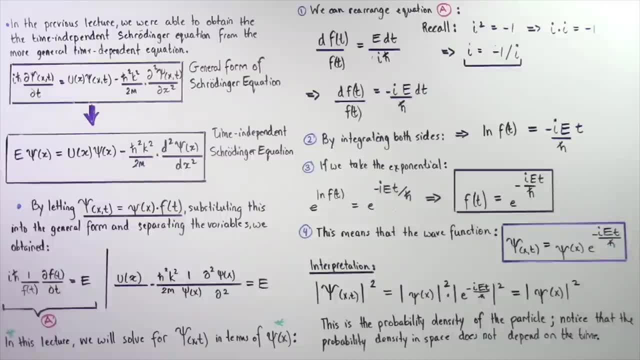 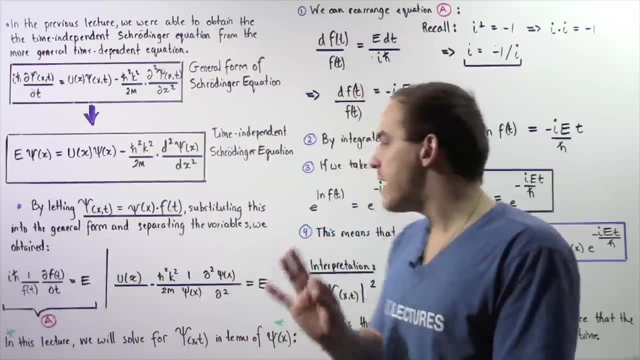 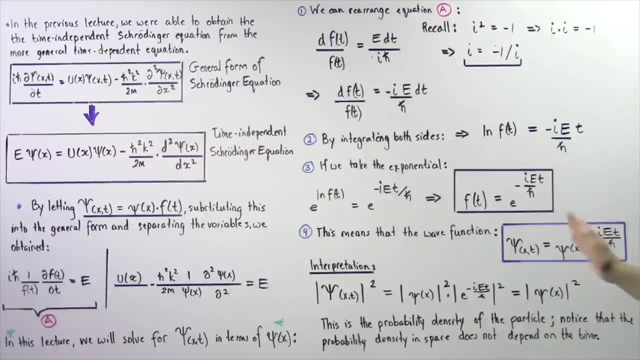 we play around with it and we get rid of the negative, i well, in that case that will produce some type of value that is, in fact, physically measurable. Now, what we can do is we can take the square of the absolute value of both sides. So if we take the square of the absolute value, 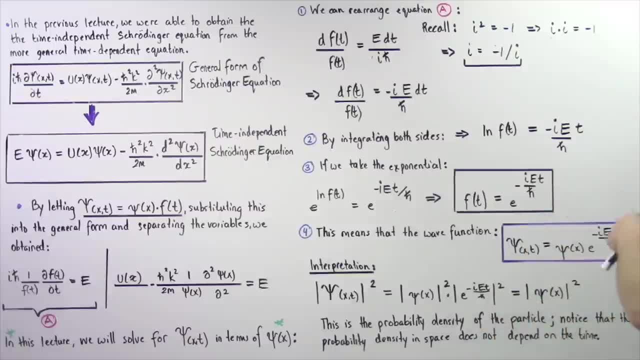 of the left side. that means we have to take the square of the absolute value of the right side, and that's exactly what we do Now. notice: the absolute value of e to the negative i e t divided by h bar is simply equal to 1, and 1 raised to the power of 2 is equal to 1.. So this quantity. 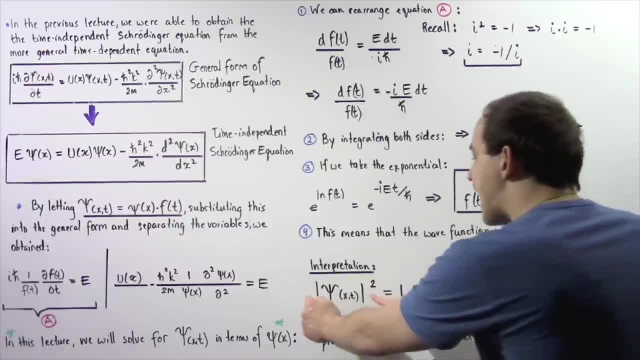 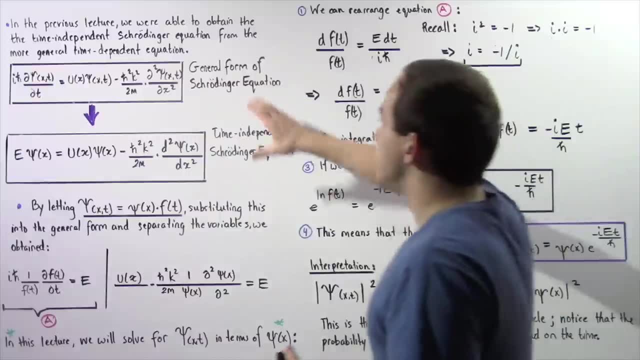 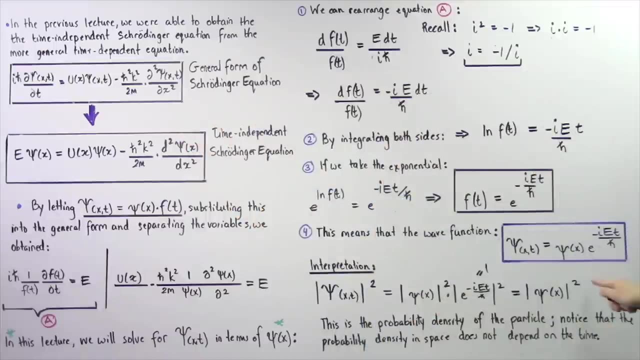 disappears and we see that the square of the absolute value of the total wave function that depends on position and time- that appears in the general form of the Schrodinger equation, the time-dependent equation- is equal to the square of the absolute value of the wave function. 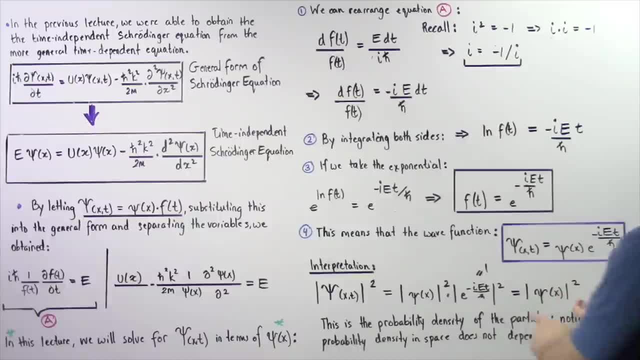 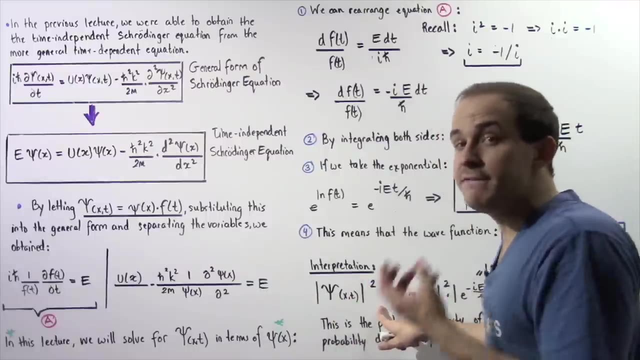 that only depends on x and does not depend on time. So this is what appears in a time-independent Schrodinger equation. So what exactly is the importance of this? What is the meaning behind this physically measurable, physically meaningful value? Notice that now we're not dealing with 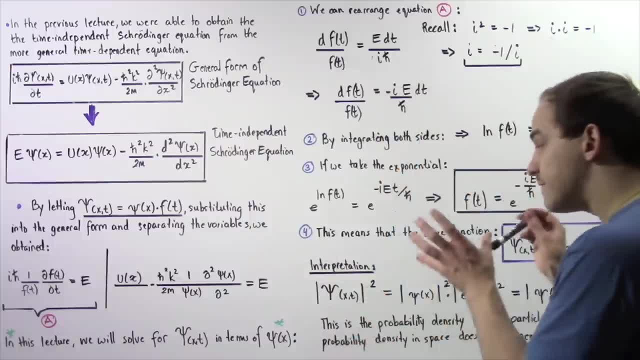 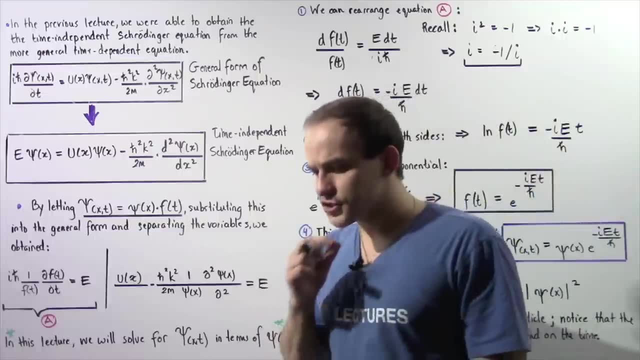 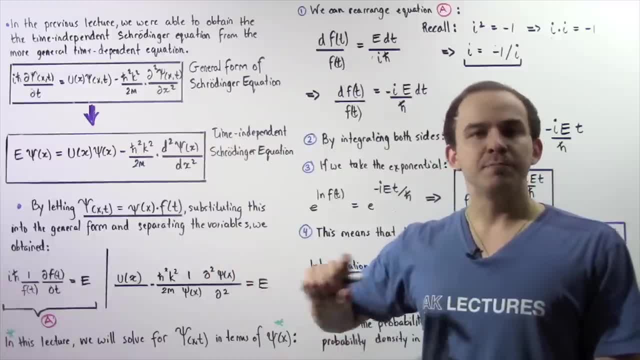 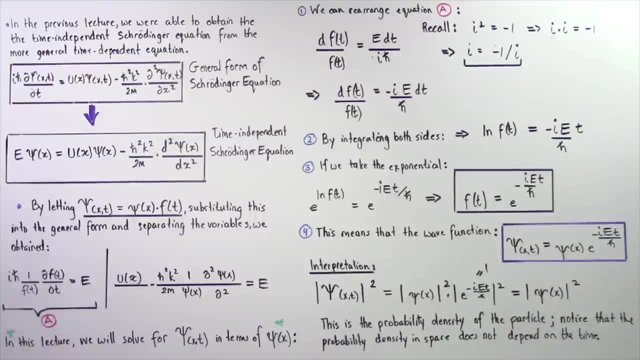 of finding our electron along any position along the x-axis. So this is known as the probability density of our particle. Now notice, because this is the probability density of our particle. this is the same exact thing as this, and the right side of our equation does not actually depend. 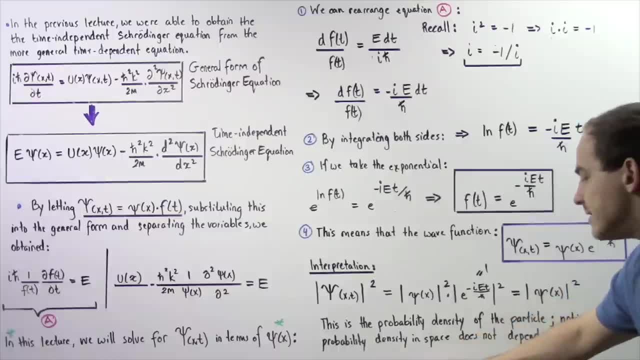 on time. that means the probability density of our electron, our particle in space does not actually depend on time. So what exactly is the meaning behind this idea? So let's suppose we have the following region of space. So notice, we're dealing with a two-dimensional region in space. 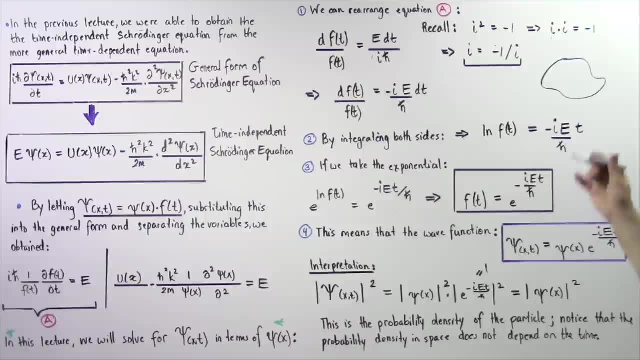 So let's suppose that we calculate, we know that the probability of finding an electron in this region is basically 20%. So we know, we calculate this and the probability of finding an electron in this region is 20%. So what exactly does this statement mean? So, because this is equal to this: 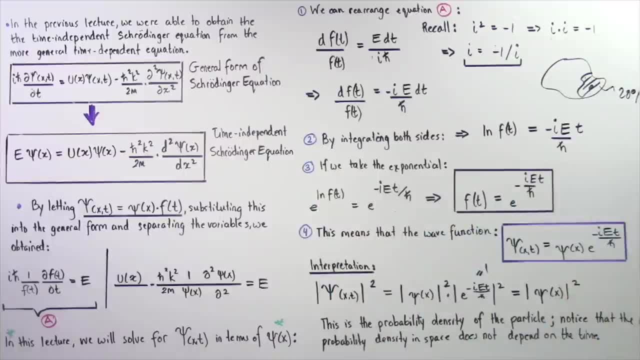 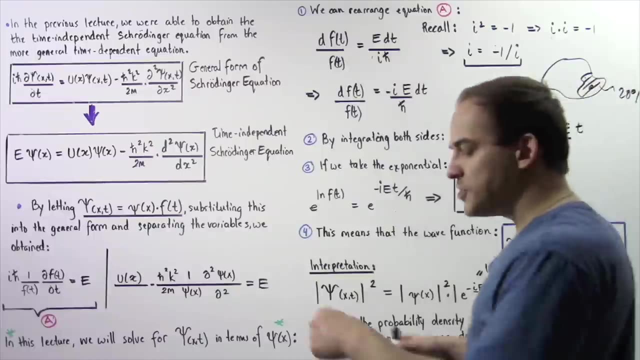 and this does not depend on our time. that basically means it doesn't matter what the time is. our probability of finding the electron in this region of space will always be the same. It will always be 20%. So basically it doesn't mean if we check now or in an hour. 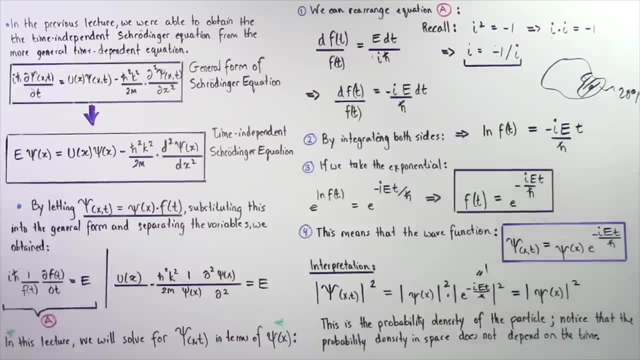 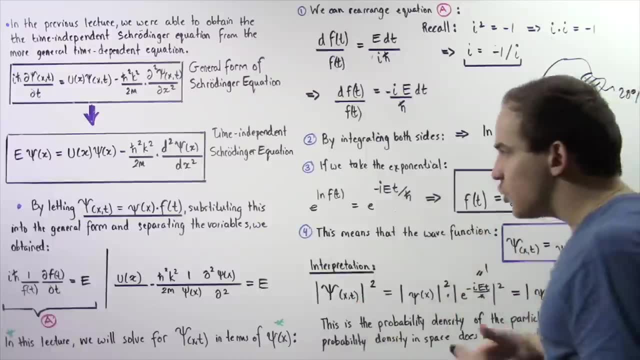 the probability of finding that electron in that region will always be 20%. That's exactly what we mean by the following statement, So let's review what we just discussed. So in the previous lecture, we basically used the following statement: So let's review what we just discussed. 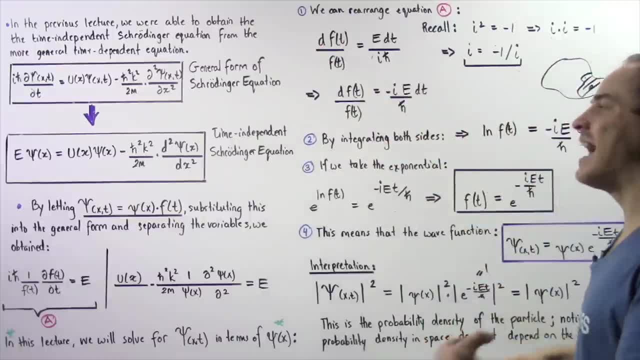 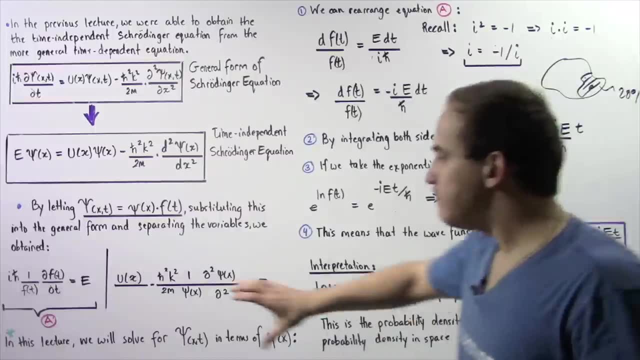 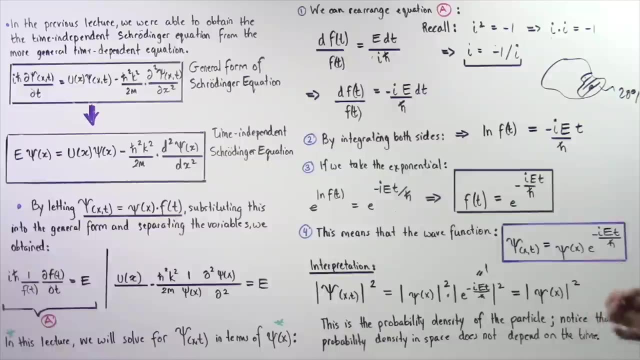 the general form of the Schrodinger equation, known as the time-dependent equation, to solve for the time-independent equation- And in this lecture we basically used equation a to determine what the probability density is- The probability density is basically given by the following equation: If you take this and square it and square the absolute value, that gives us the